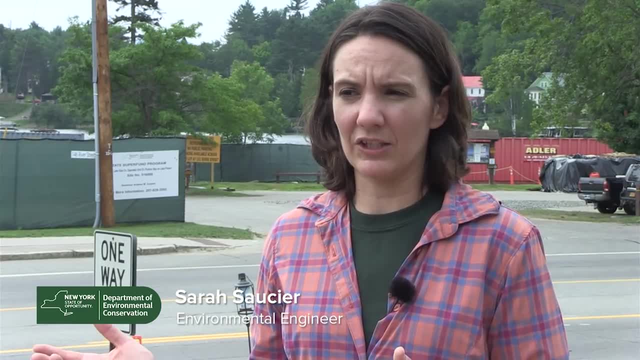 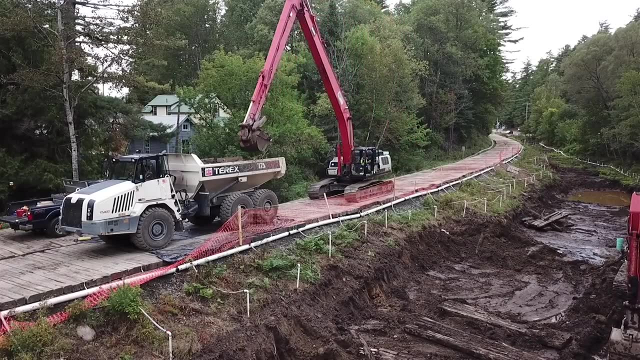 SARAH SOCHE. We have environmental controls out here to make sure that we're not spreading the contamination anywhere, that we're actually cleaning things out. So I just walk around and make sure all the environmental controls are up and running and that they're working. 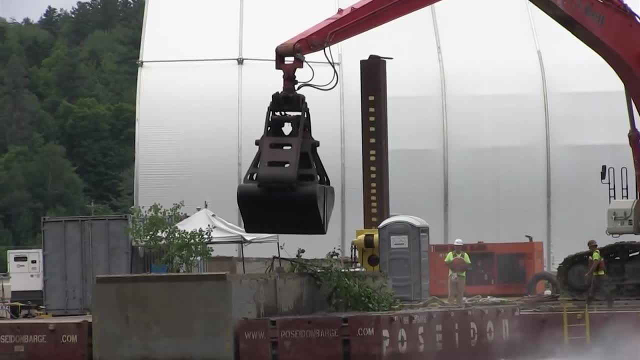 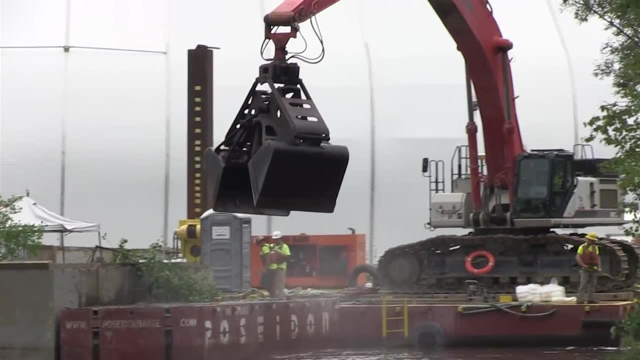 and that they're up to standards. HARI SREENIVASAN, Contaminated sediment can have an odor, So Soche and her team are also responsible for ensuring odor controls are in place and that no dust leaves the site. All major construction activities are scheduled to be completed by the end of the year. 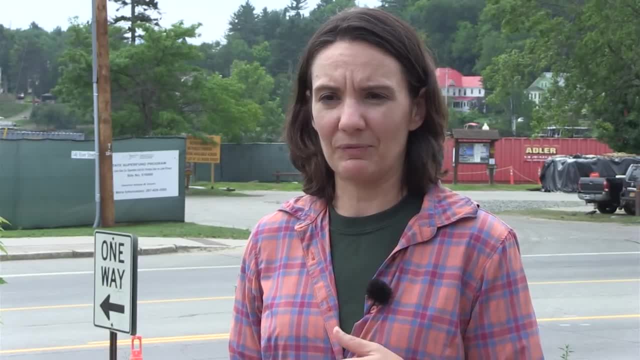 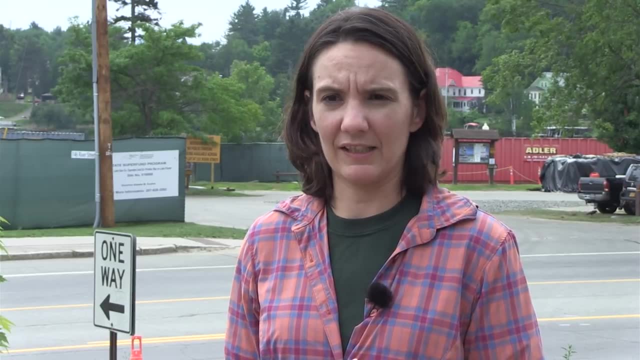 SARAH SOCHE. We might have to come out in the spring to do some restoration activities, do tree plantings, restore Brandy Brook with grasses and things like that. But the bulk of it will be done by the end of the year. 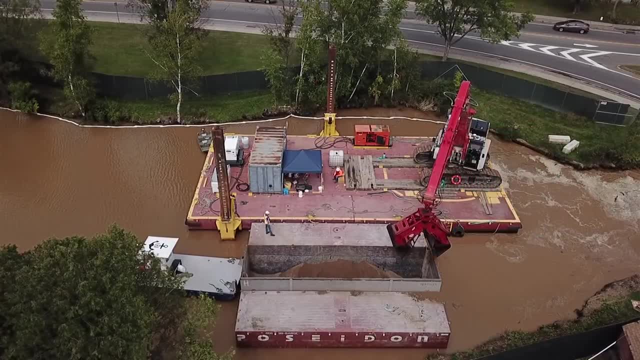 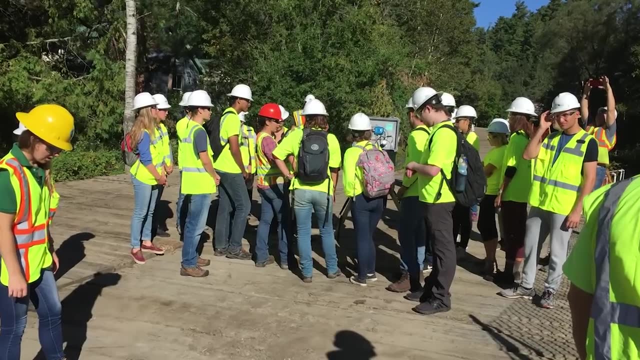 HARI SREENIVASAN Soche says so far feedback from the public has been extremely positive. as residents have expressed, they're pleased with the cleanup of the Brook and the Bay. Students from a local high school and Clarkson University reached out to DEC about touring. the site And DEC staff said they're happy with the clean-up. HARI SREENIVASAN Soche says so far feedback from the public has been extremely positive. as residents have expressed, they're pleased with the clean-up of the Brook and the Bay. Students from a local high school and Clarkson University reached out to DEC about touring the site. HARI SREENIVASAN Soche says so far feedback from the public has been extremely positive. as residents have expressed, they're pleased with the cleanup of the Brook and the Bay. 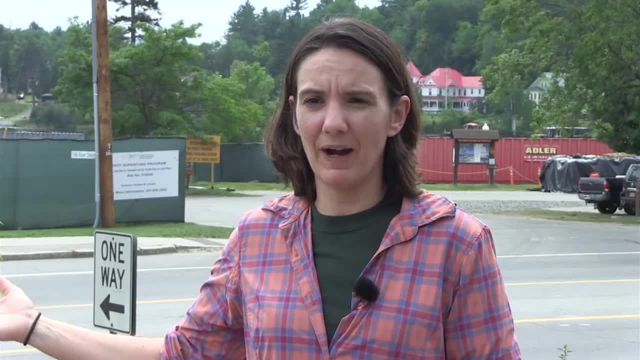 Students from a local high school and Clarkson University reached out to DEC about touring the site. HARI SREENIVASAN Soche says so far feedback from the public is extremely positive, as residents have expressed, they're pleased with the cleanup of the Brook and the Bay. 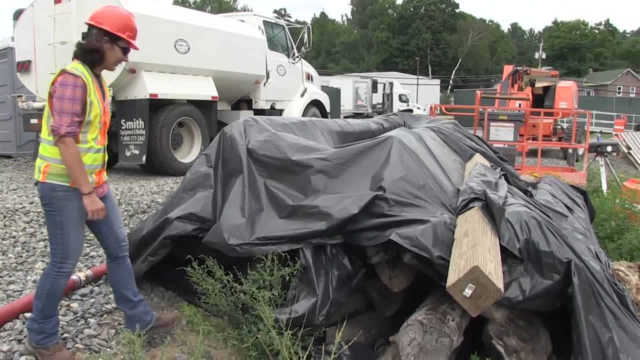 Students from a local high school and Clarkson University reached out to DEC about touring the site. HARI SREENIVASAN Soche says so far feedback from the public has been extremely positive. as residents have expressed, they're pleased with the cleanup of the Brook and the Bay. 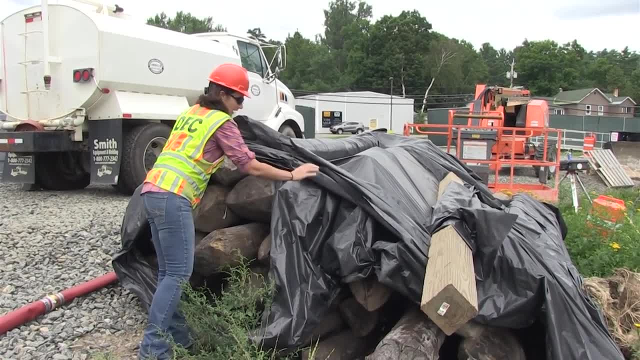 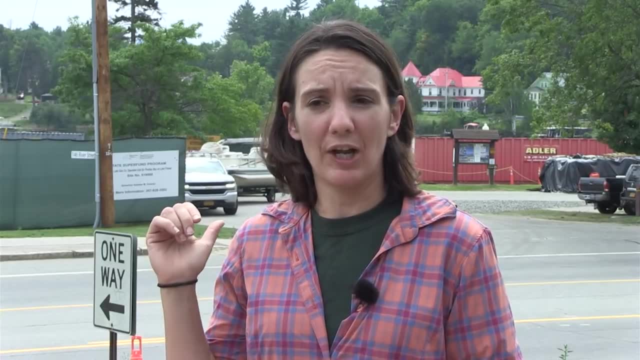 Students from a local high school and Clarkson University reached out to DEC about touring the site and it's really. it's a historic part of this community and the Adirondack experience at the museum in Blue Mountain Lake found out about this, while our public participation specialist actually. 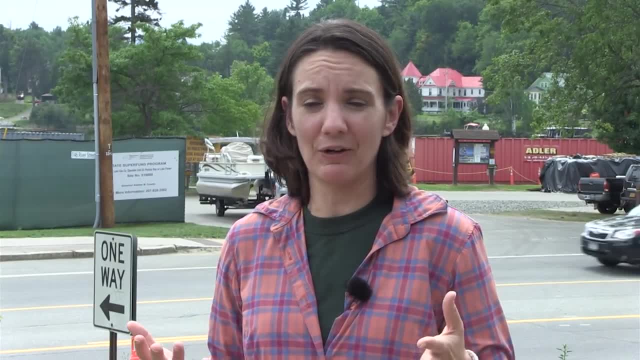 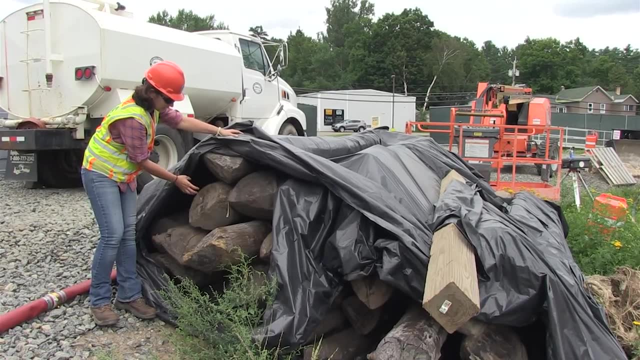 reached out to them and the local historic society and they're both like, really excited about these logs because it's a big part of the history here. so we're working with them to clean up the logs, to save them, so it can become a part of the collection. 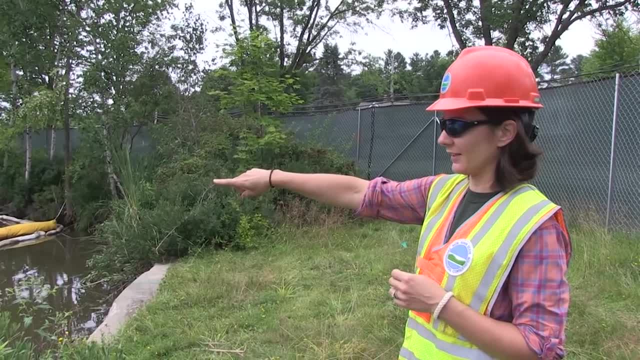 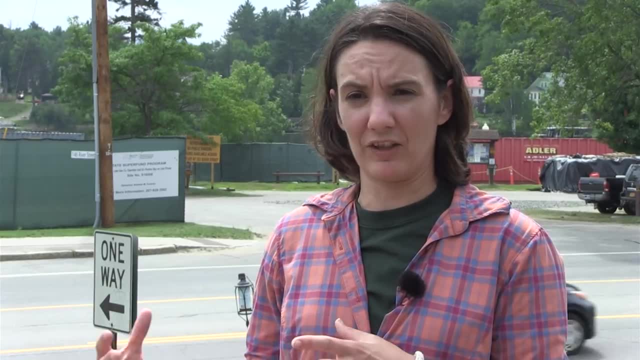 For Soche. this is not just a job. she's got a personal stake in what she does. After working in the private industry, I decided that I really wanted to work on the right, the public side of things, the regulatory side of things, maybe working with the public a little bit more.